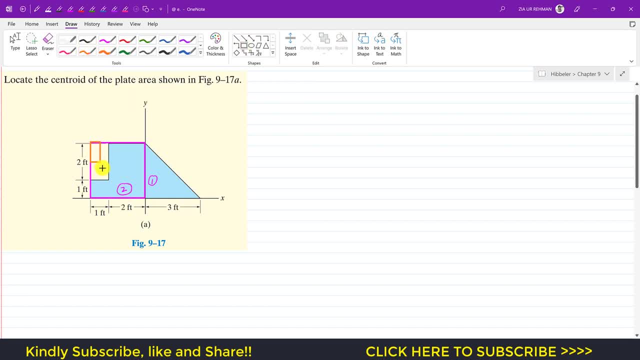 and the third segment can be this: We consider this as a negative area: this rectangle, This is, let's say, third segment. So to find the centroid, we need to develop a table which would have the segments, then the area of each segment, then x bar- sorry, x tilde. 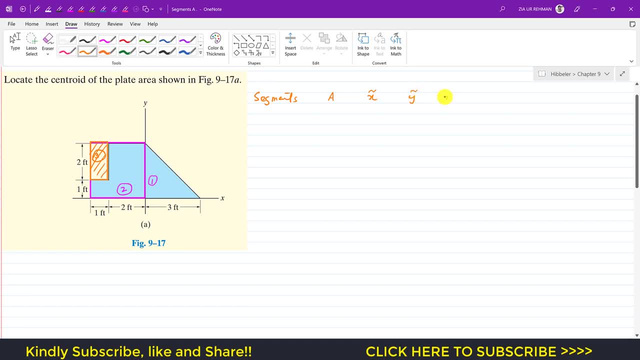 Then y tilde, then x tilde times the area, then y tilde times area. So, since we know that if you want to find x bar of the centroid, then x bar is always equal to the summation of x tilde times area divided by the summation of the area. 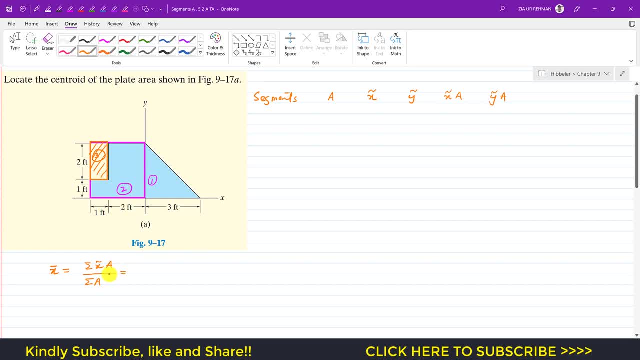 So what does this mean is that, since we are considering three segments, so then this will be equal to x tilde 1 times the area of six segments. So this will be equal to x tilde 1 times the area of six segments. 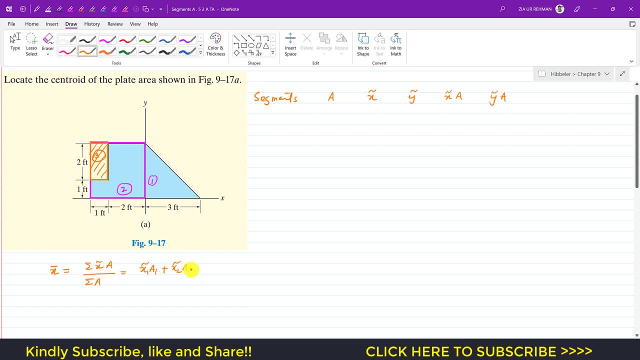 So this will be equal to x tilde 1 plus x tilde 2, multiplied by area 2 plus x tilde 3 and multiplied by area 3, and then this will be the summation of area 1 plus area 2 plus area 3.. 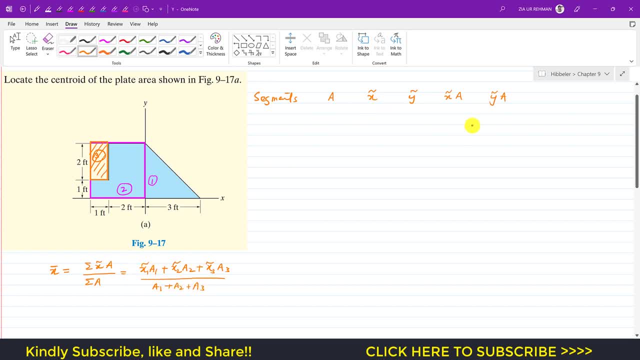 So for this we develop this table and then we add up the x tilde times a for each segment and the y tilde times a for each segment, and that gives us the x bar of the centroid and similarly, if you want to find the y bar, 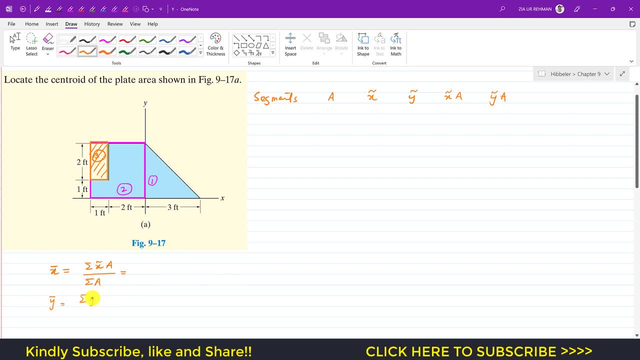 then y bar is equal to the summation of y tilde times area divided by the summation of area. Now we have to locate the centroid of each of these three segments, right? So let's say that this is, this is our segment one. 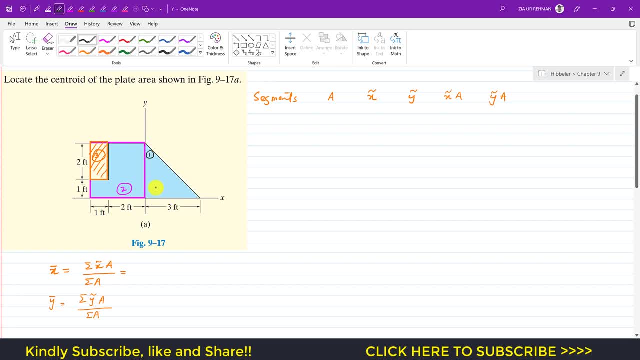 So the centroid of this triangle will be somewhere here and its location from the x-axis will be this distance From the x-axis, this will be y tilde and this distance from the y-axis, this will be x tilde. This is x tilde, or we can say that this is x tilde 1 and y tilde 1 for segment one and, as we know, 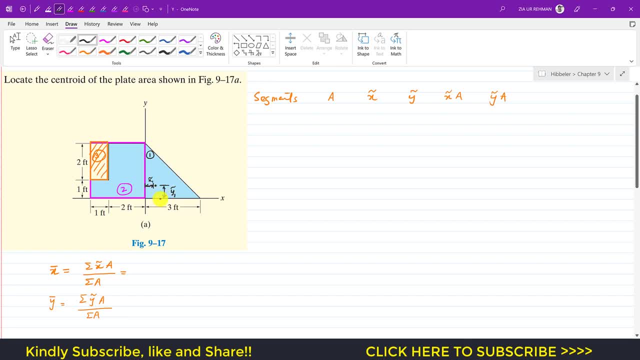 that for triangle, the distance of the centroid from the base is: this is equal to the height divided by three. so the height of this triangle is three feet right. so three divided by three is one. so y tilde is one. Similarly, x-tilde will be equal to this distance, this height divided by three. so again, 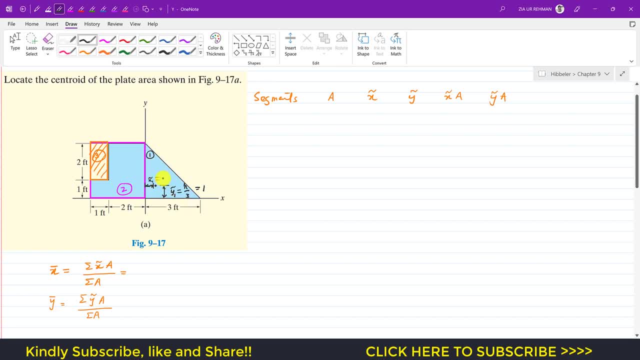 for this x1 tilde, the base is this, so then this is the height, and then this is 3 divided by 3, so this is 1.. So now from this we can say that the centroid of this triangle is at a distance of from this origin. 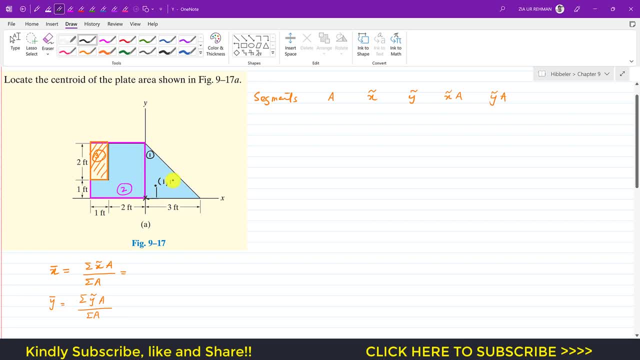 it is at a distance of 1 feet and then it is at a distance of 1 feet, so this is one n 1. the location of this is 1: 1, so we can write that segment 1, the area of the segment 1, since it's a. 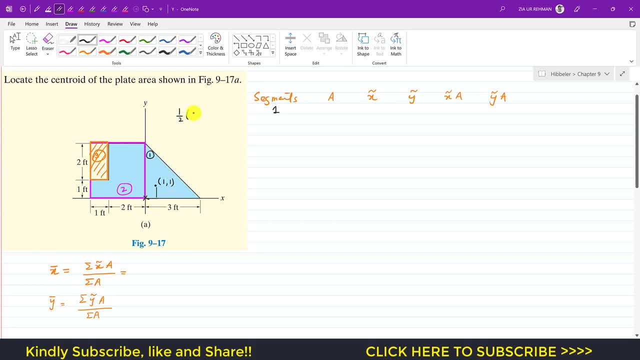 triangle, so its area will be 1 divided by 2, and base is 3 and height is 3 as well, so this is 3 into 3, 9 divided by 2, so this is 4.5 feet square, so the area unit is feet square, and similarly as 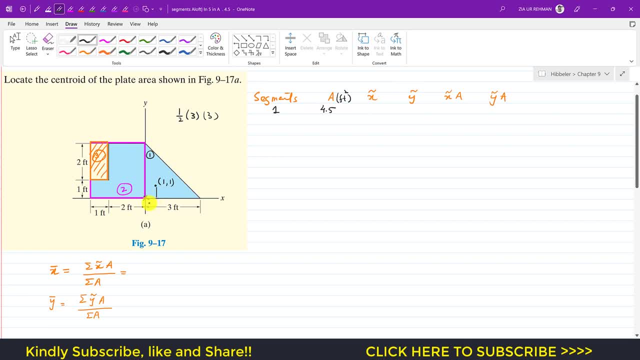 we have determined that this is x tilde, so x tilde is 1. this is 1 feet and this is also 1 feet, so this is 1, and y tilde is 1 as well, so x tilde times a. now this is 1 into 4.5, so this is 4.5. 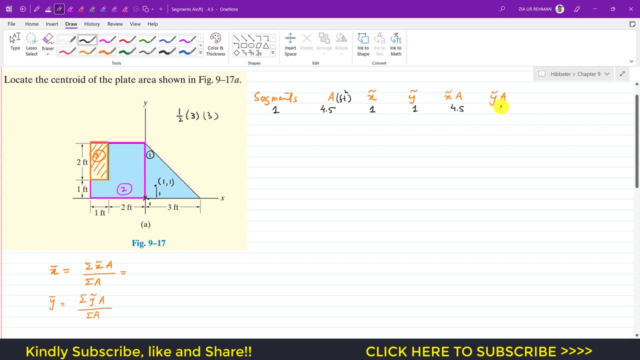 and again y tilde times a. so this is 4.5 again and the unit of this will be in feet. this will be in feet as well, and this will be feet into feet square. so this will be feet cube and, similarly, this will be feet cube as well. 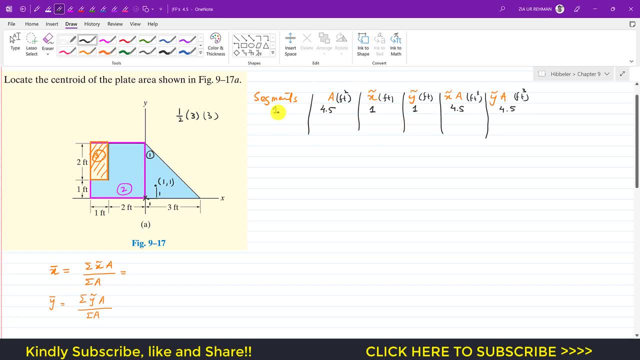 so now for segment 2. let's say that for segment 2, now, this is our segment 2, this square. so the area of this square is 3 into 3, so there is 9 feet square and it's its centroid will be at its. 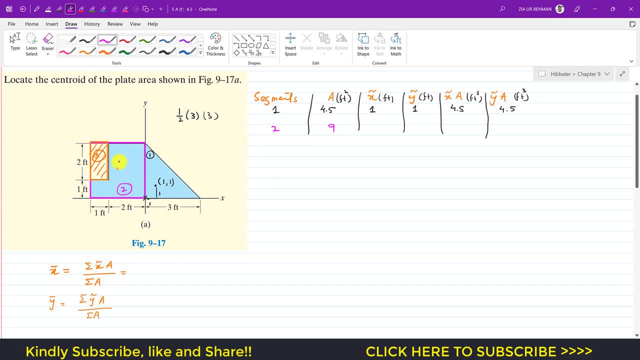 geometric center. so this, let's say that this is the centroid of this segment. 2, this is c2, so its location from the origin, in from the y-axis, is: this: distance will be half of 3. it is 2 plus 1, 3, so this is 3 divided by 2, so this is 1.5, and similarly, 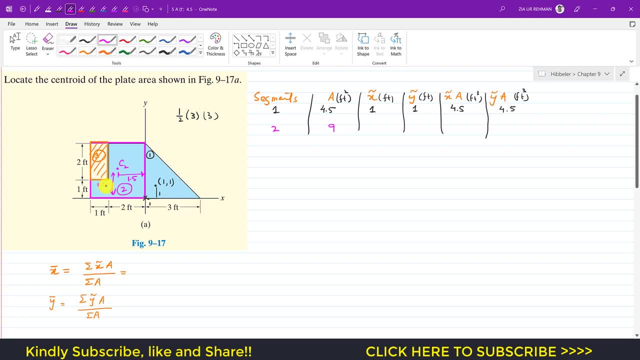 from the x-axis. this distance will be 1.5 as well. so this will be x tilde for c2. this is: this will be the distance from the y-axis. is is x tilde for 2 for segment 2 and this will be y tilde for segment 2. so we can write that x tilde for segment 2 is 1.5 and y tilde. 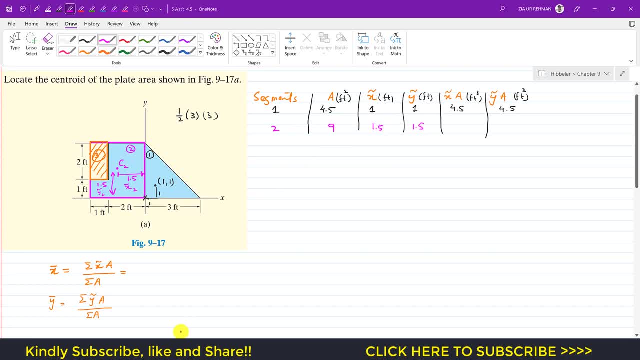 for segment 2 is 1.5.. 2 is 1.5, and 1.5 into 9 is 9 multiplied by 1.5. this is 13.5, this is 13.5 and this is also 13.5. 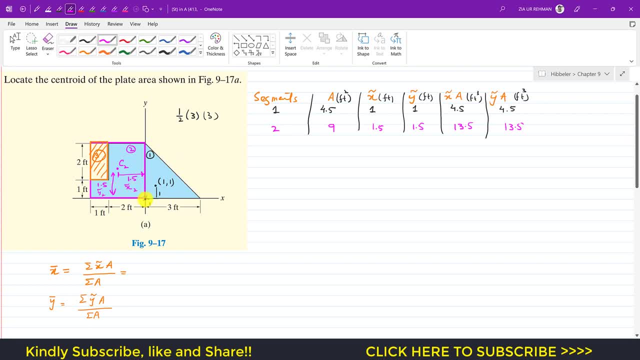 but remember that in this direction this will be, since this is the origin. so this will be minus 1.5, remember. so this means that x tilde 2 is minus, so this is minus, so this is 9 into 1 minus 1.5, so this will become negative as well, and this one is positive. remember now the segment 3. 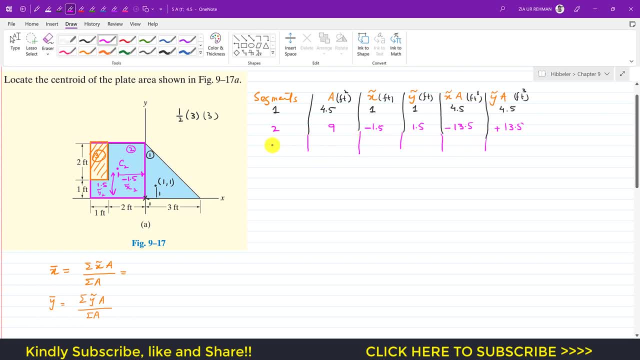 for segment 3. that is the negative area. we have to consider it. we have to subtract it so that area is: this is 1 feet, so 1 by 2 is 2 feet square, so 2 feet square, and we have to subtract it. this is: 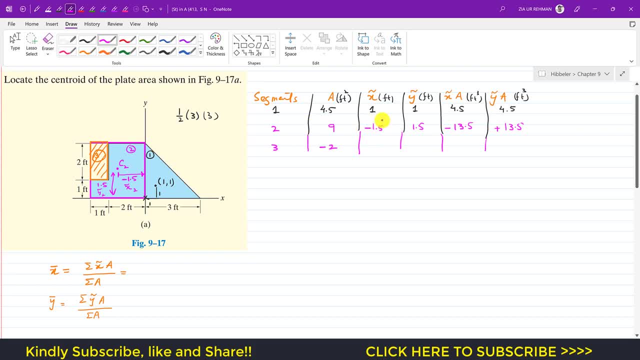 the negative area. this is not included, so and x tilde will be. the location of its centroid will be somewhere here, so it is geometric center. this is segment 3. so now the location of its centroid from the origin is this distance will be. this distance is x tilde for segment 3 and this will be 2. 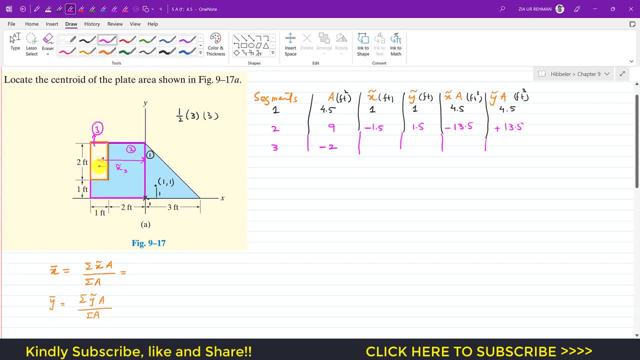 plus half of 1 feet, so from here to here this is 1 divided by 2, so this is 0.5. so 2 plus 0.5, so this will be 2.5. so x tilde for segment 3 is: 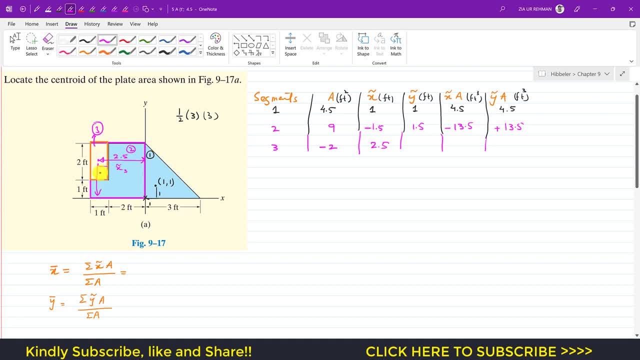 2.5 and similarly this will be y tilde, so y tilde, y tilde will be 1 and the half of this, this from here to here. this will be 2 divided by 2, so that is 1. so 1 plus 1 is 2 feet, so this is 2. 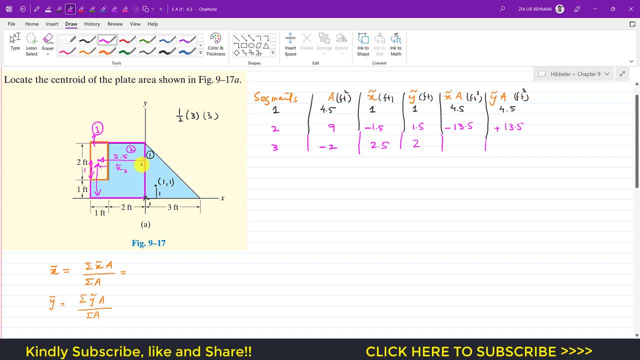 and again, as we can see that this x3 is in the negative x direction, so that will be minus minus 2.5. so now minus 2.5 into minus 2, so that will become plus 5, and this is 2 into 2 is minus. 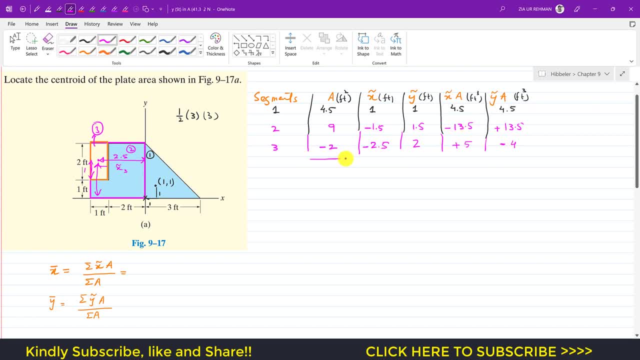 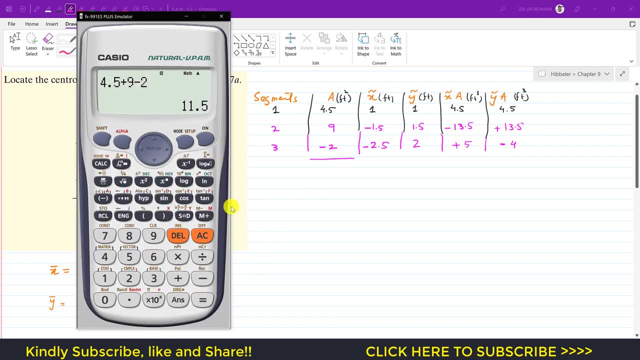 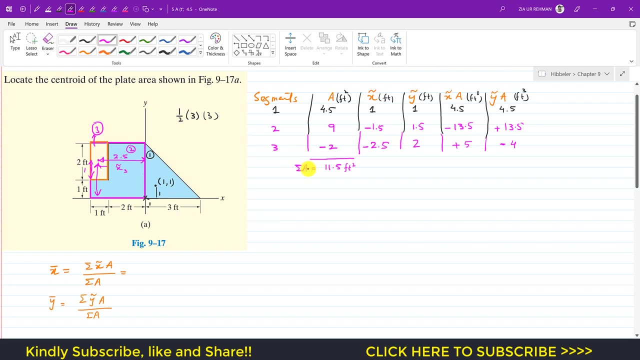 4. so now we have to add up: this area is 4.5 into 9, 4.5 plus 9 minus 2. this gives us 11.5, 11.5 feet square. this is the summation of area of each segment. now the summation of x tilde times a. so 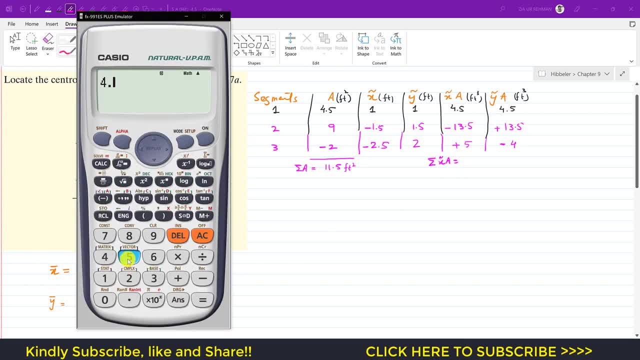 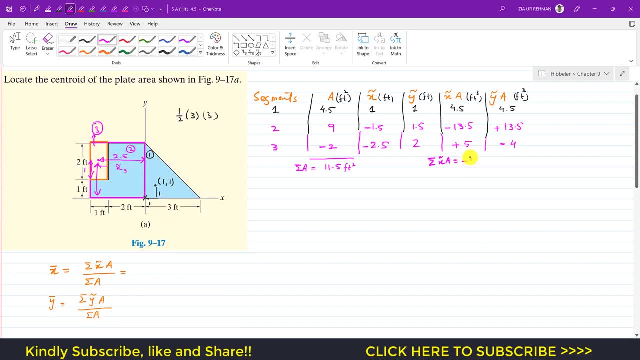 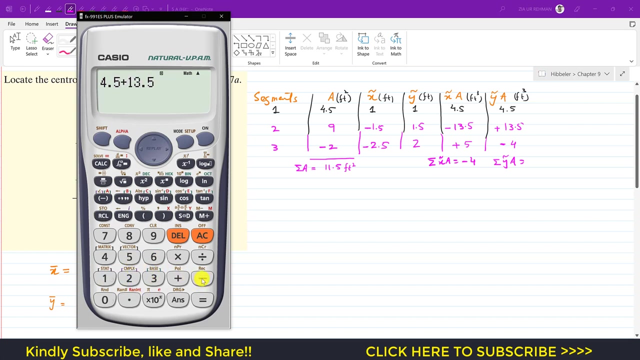 we have to add up this: 4.5 minus 13.5 plus 5. this gives us minus 4. this is minus 4 and the summation of y tilde times a. so we have to add up this. so this is 4.5 plus 13.5 minus 4. this gives us: 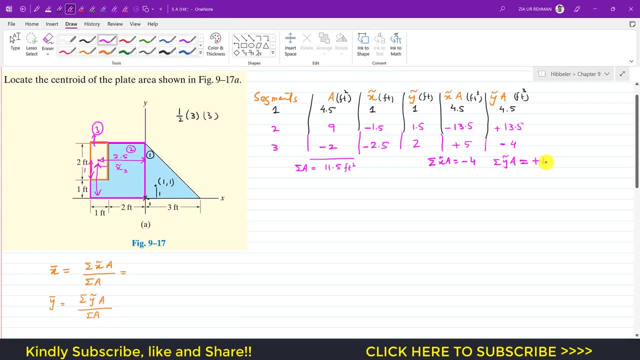 14. so this is plus 14. this is equal to plus 14. and now we know that from this equation we know that X bar is equal to The summation of x tilde times a is minus 4 divided by the total area. This is divided by 11.5.. 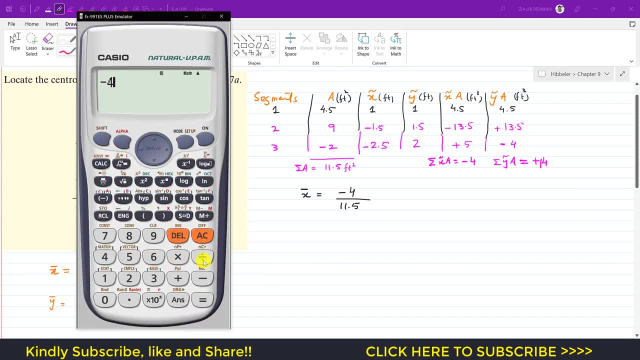 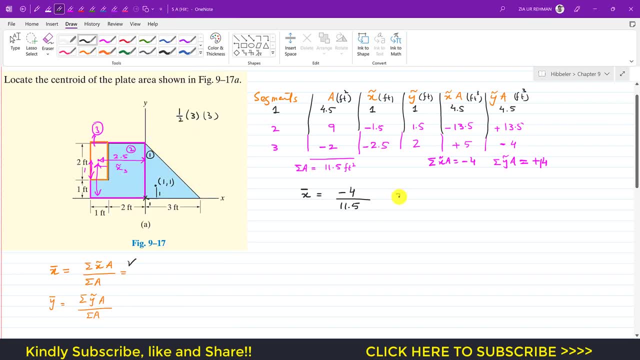 So minus 4 divided by 11.5.. So this gives us minus 0.348.. So x bar is minus 0.348 feet. Similarly, y bar is equal to the summation of this, That is, plus 14 divided by total area, which is 11.5..